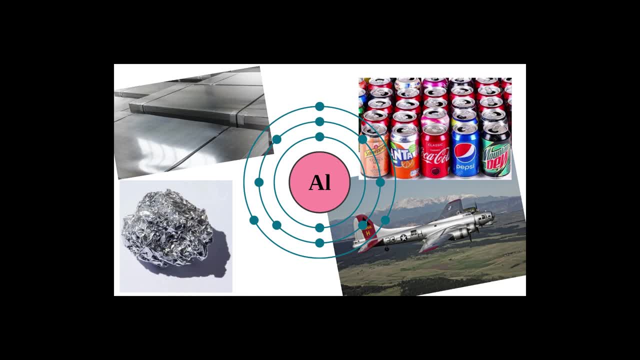 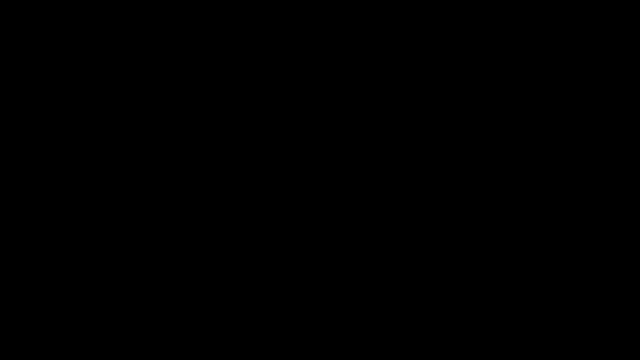 Aluminum. It's aluminum. I don't know what you expected, because this is so Silicone. It's used for making chips. Phosphorus Sulfur. In the recording I- I sound like I'm at gunpoint, Guys. please forgive me this. I'm not at gunpoint. that you know of. 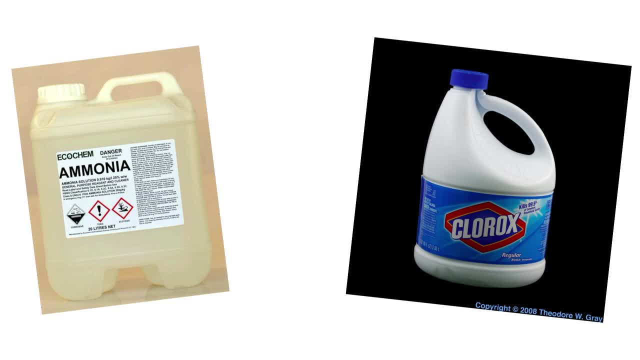 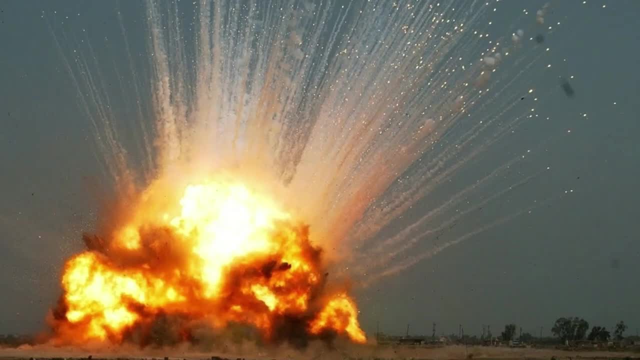 Chlorine. Mixing ammonium and bleach does not make mustard gas Gives you chloramine. I mean you still shouldn't do it. but- Argon- It's used to make light bulbs. Potassium- You know what potassium is used for. That's right. 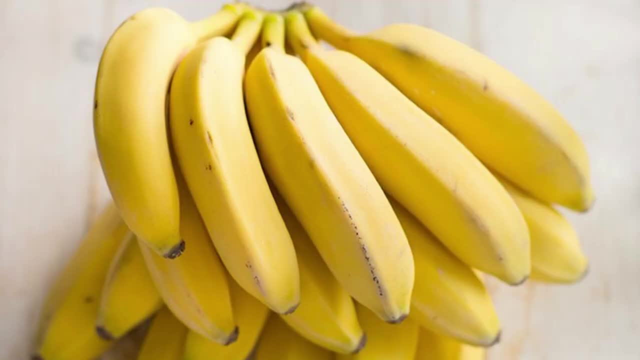 Explosives Plus. I guess you need it for your body, but you know that's neither here nor there. Calcium- Ooh, Mr Bones. Scandium, Alloyed bikes. Titanium- Not alloyed bikes. Vanadium. 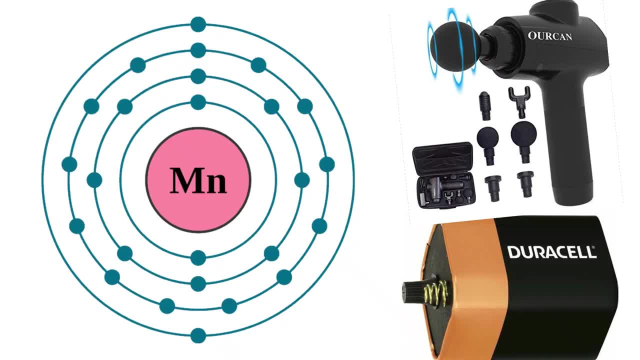 Some- Sometimes alloyed bikes. Chromium- Hey, your grandpa knows that one. Hey, your mom knows that one. Iron- It's iron, What-. What else do you think it is? Cobalt, Goblins, Nickel: Two loonies and a toonie get you half a pound of this stuff. 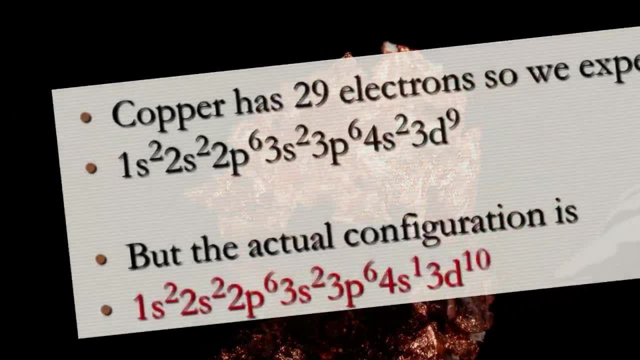 Copper You existing gives me pain Whenever I do the electron configuration. guys. it sounds nerdy, but trust me, keep on track. This is a little secret for zinc. Don't melt your pennies down and sell the zinc for profit, guys. 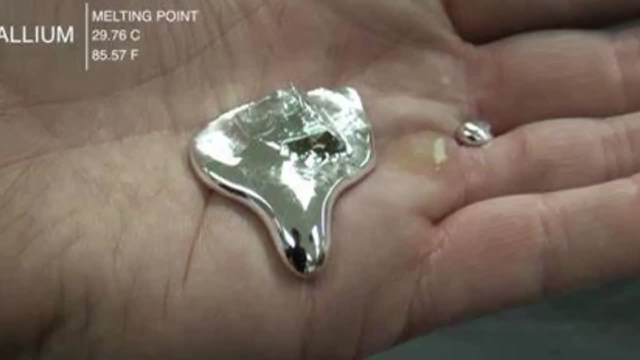 Guys, guys, don't do that. I'm telling you guys, not to Gallium. Gallium is the safer version of mercury. Does anyone else remember the gallium challenge? Like I swear, I bring it up to anybody and they say they've never heard the gallium challenge. 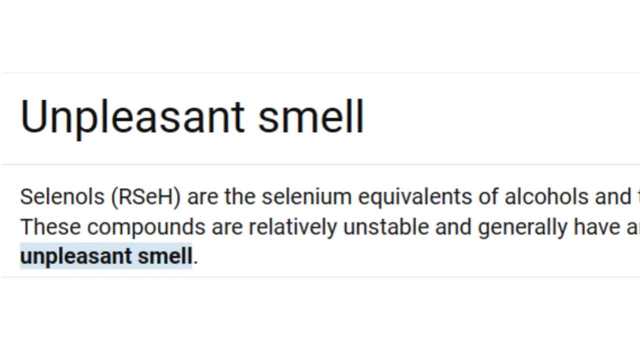 Germanium, Diodes, Arsenic, Poison, Selenium- This one makes you smell bad. Oh, it's in nuts, so Bromine, Flame, retardant. What did you call me Krypton? No, not the planet. 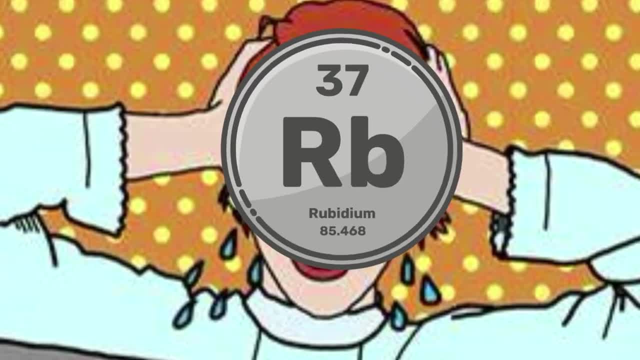 It's still pretty dope as hell. Rubidium, Unlike lithium, his meltdowns would probably cost you a finger. Haha, I'm just kidding. You guys probably wouldn't survive. Strontium, Fireworks, Yttrium. 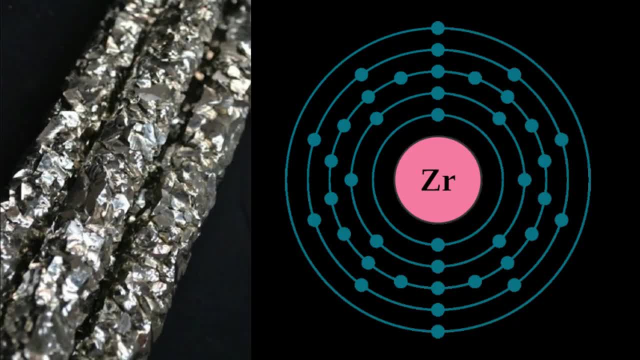 Yags, Yes yags. Yttrium, aluminum garnet, okay, Zirconium, Cool name. Oh yeah, I guess he can kind of absorb electrons and escape the hellish pits of a nuclear reactor, Niobium. 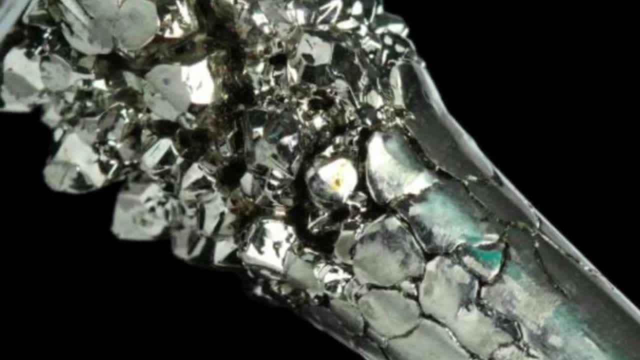 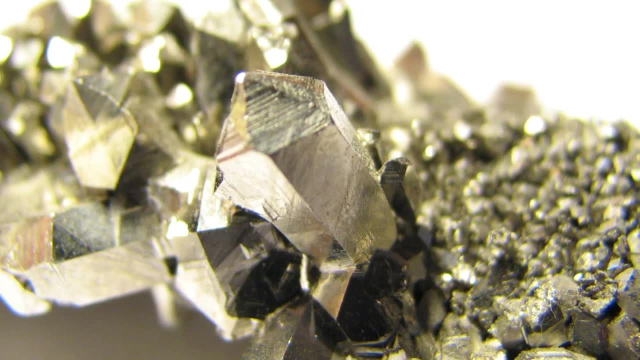 I'm gonna say it: This one's crystals are prettier than bismuth. You stupid pick-me-bit, You wanna buy a crystal for your girlfriend, Or Who am I kidding? Do you really have a girlfriend? I would recommend niobium instead of bismuth. 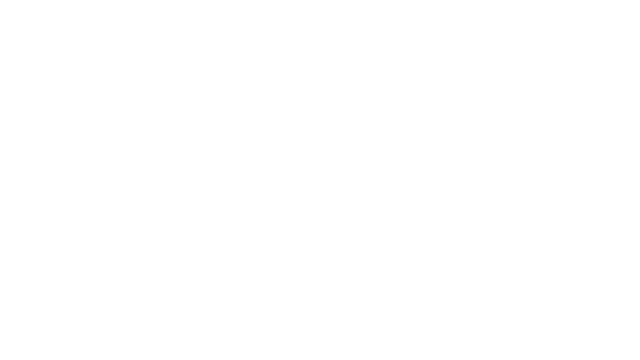 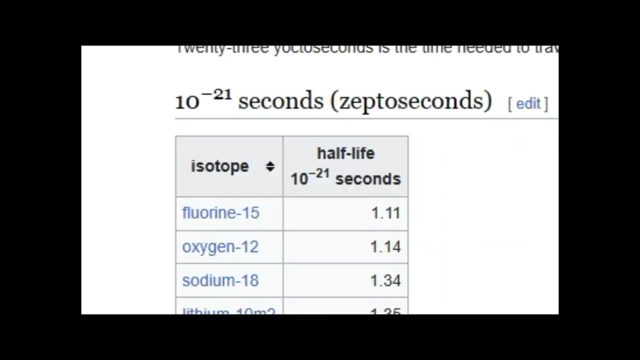 Higher melting point, Prettier colors. I mean, look at this. Molybdenum, That's the natural element name Important in steel manufacturing Technetium. Now this is the first radioactive element that we see Other than the isotopes. you pretentious nerds. 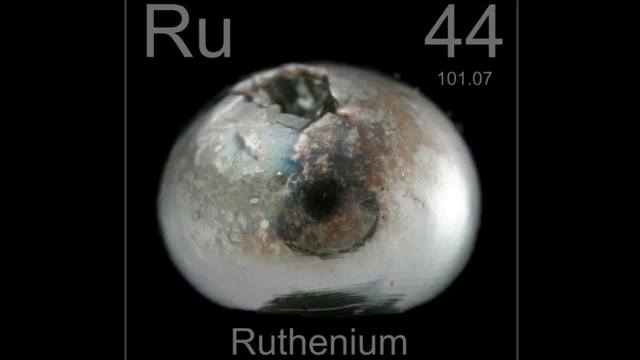 All right, don't correct me. So it's pretty useful in bone marrow and liver imaging. Ruthenium Jewelry, Rhodium Jewelry. Also Cadillac converters, Palladium Jewelry. Also ceramic capacitors. Silver Please, It's silver. 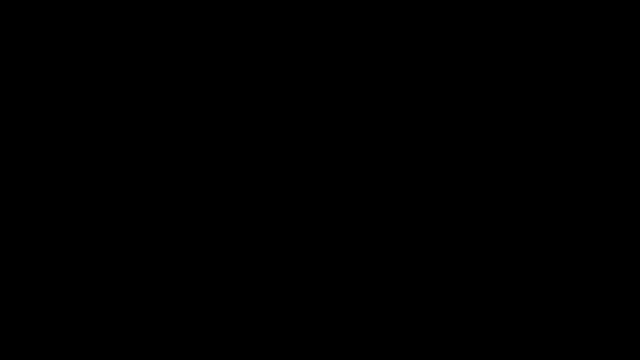 You already know this one. All right Cadmium, This one's basically diet lead Indium. Indium is a very soft metal, So soft that you can chew it, And I've done it before. Tin- No, Tin foil isn't made of tin. 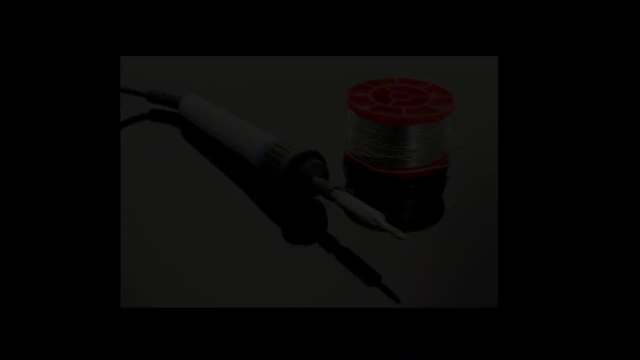 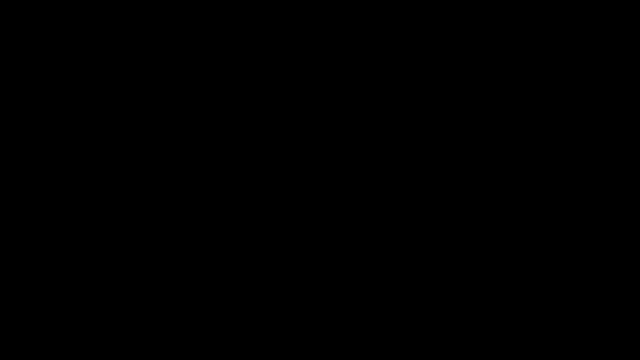 Tin cans are also not made from tin. But you know what is made from tin. That's right, The big Buddha Antimony. Very pretty color solutions, Very not so pretty health conditions, Tellurium- This one's used in optic fibers, but also touching this pure metal will make you smell. 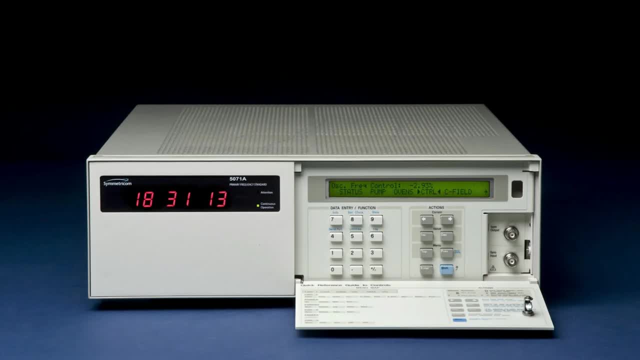 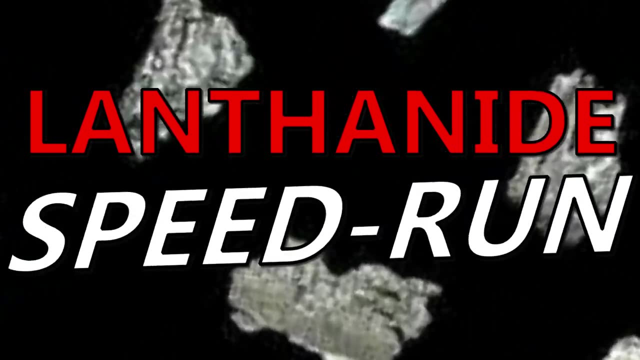 Iodine. This one's both good and bad for you. Xenon, Carlites, Cesium, Atomic Clocks, Barium- Fuck you All right. So now we've reached this awkward bit of the periodic table. So you know, let's get ready for the lanthanide speed run. 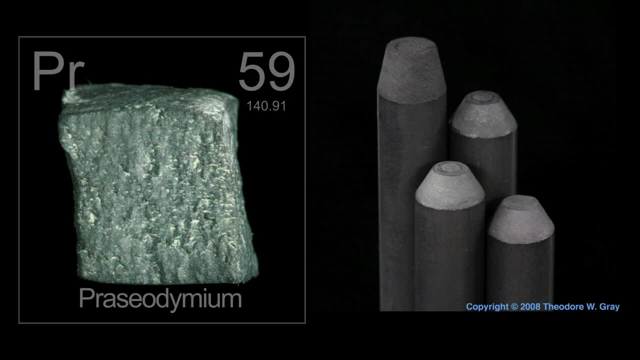 Lanthanum Lighters, Cerium Ulcer lighters, Praseodymium Alloys, Neodymium Magnets, Promethium- Useless paint, pigments and batteries. Cimmerium Magnets too, apparently. 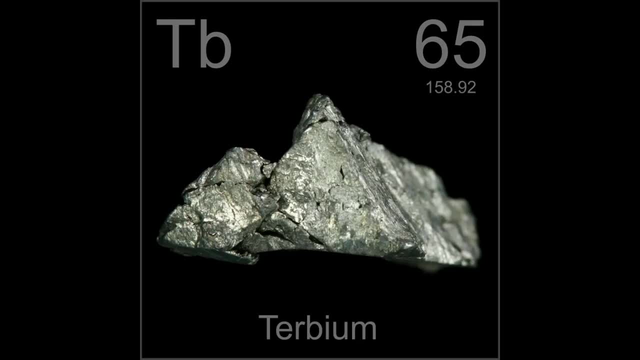 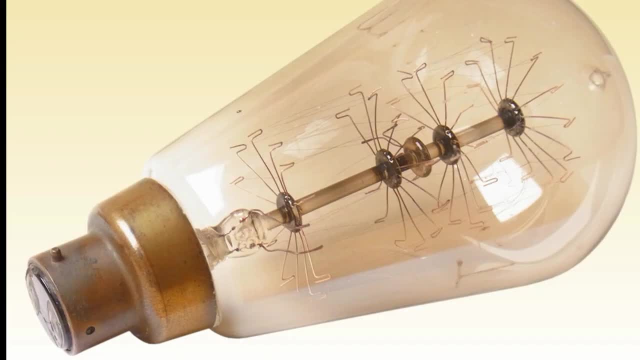 Hafnium, Badass, plasma cutters, Tantalum, White filaments, Tungsten. Yeah, He's got a hell of a high melting point. He's good at making alloys, but you know what the downside is. 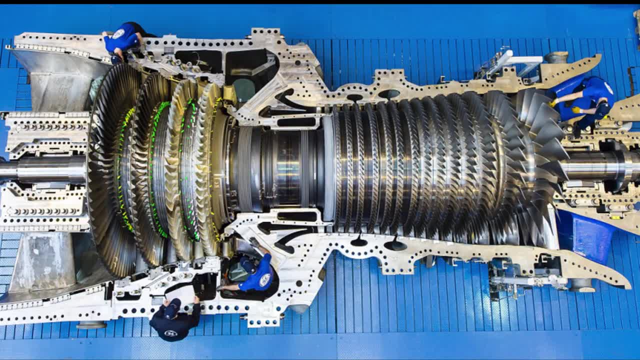 He's brittle Whoops. Rhenium: Super cool jet metal. Oh my god. Osmium- This is the densest element in the periodic table: Iridium. I don't know why people argue that this is the densest element. 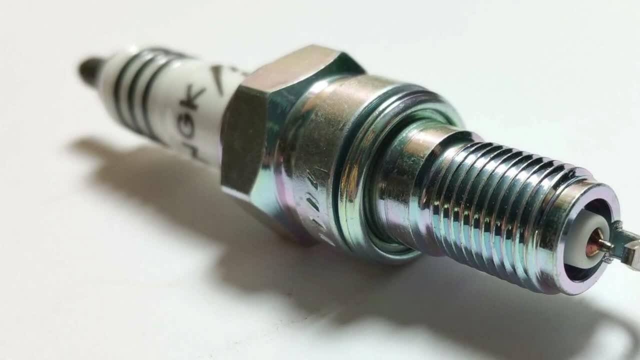 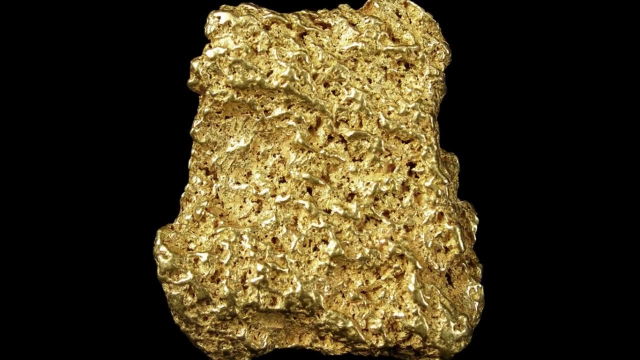 Yeah, there's a whole argument. I don't know why, But those who do argue that this is the densest element are just mentally confused. Platinum, Lab equipment, Gold, Jewelry, Alloys, Computers, Teeth, Bro- this one does the whole group project. 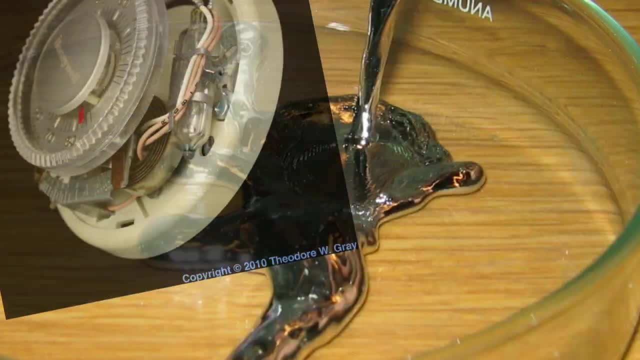 Mercury. You know he used to be useful Thermometers And thermostats- Thallium. So I got this stuff. I keep it in mineral oil In a sealed ampule, In a sealed bag, In a sealed container. 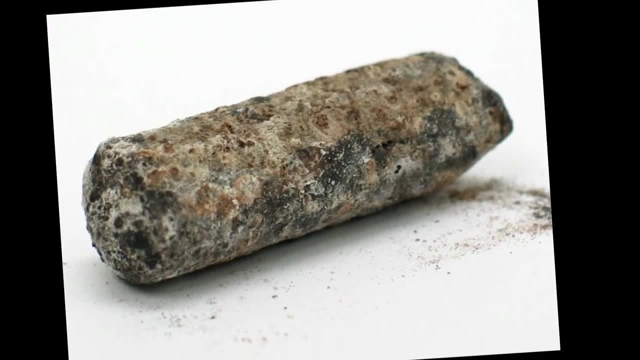 And you know what? I'm still afraid to hold it. You know why? Because it's absolutely terrifying to hold. It's super poisonous. Lead, Lead, Lead, Lead, Lead. Bismuth is the crystal girl that pretends to be ill for attention, but isn't. 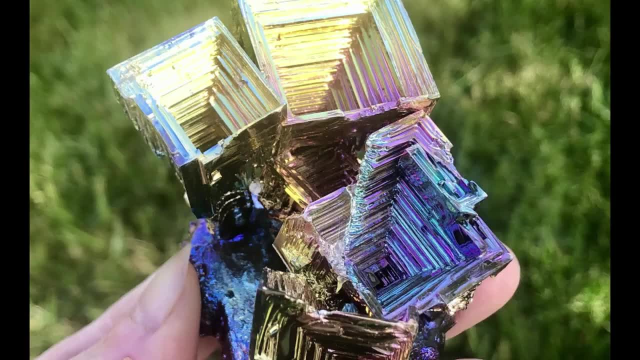 Similar to how Bismuth is slightly radioactive But not enough to harm you. Fuck you, Bismuth. People only know you for the crystals and nothing else. You are the reason I have issues with Google correcting me and showing me some random character. 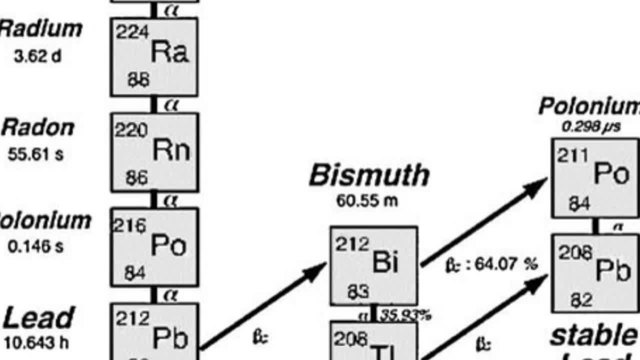 from Steven Universe. Who is that? Who is that? Oh yeah, also Bismuth is the last of the stable ones. So, uh, stuff is about to get crazy from here. Polonium Got a tux with too much static. 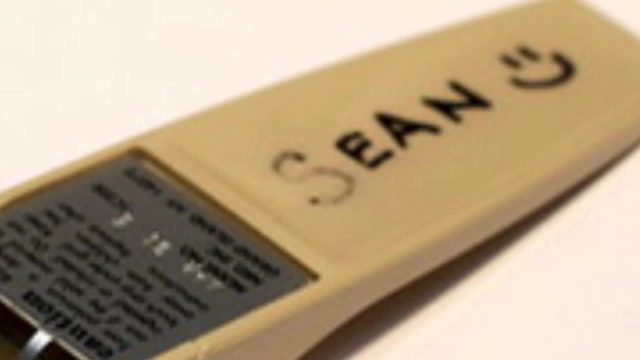 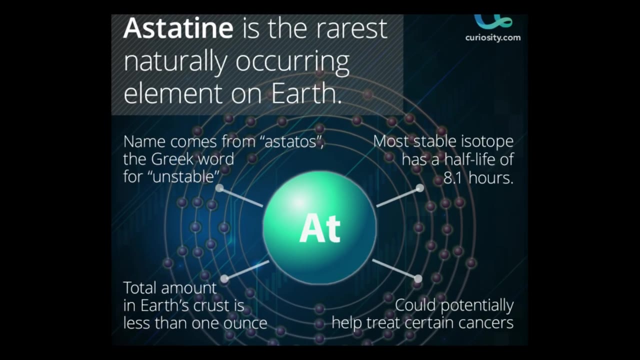 Why not use enough radiation to kill your entire family to fix the issue? That'll do the trick: Astatine. At any given moment, there's less than 24 grams of this stuff on Earth. It's almost as rare as the peace and quiet in my neighborhood when my neighbors start. 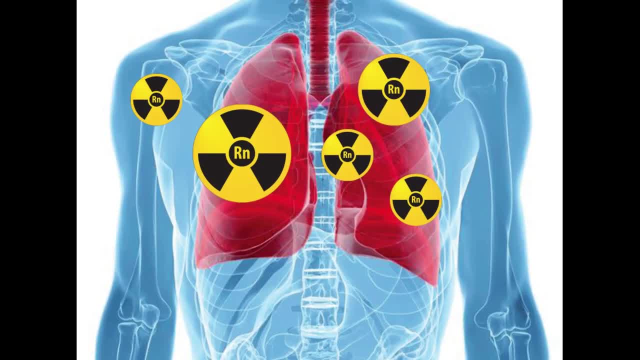 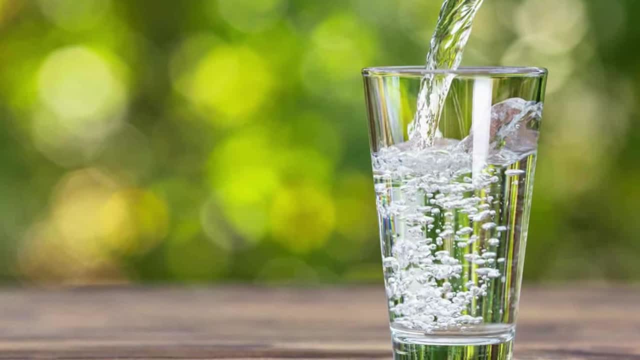 snorting grams of cocaine. Radon Want lung cancer? No, Too bad. Francium Lasts longer than my combined mental stability in an entire day At 22 minutes Radium. Hey, you want some positive energy in your water? 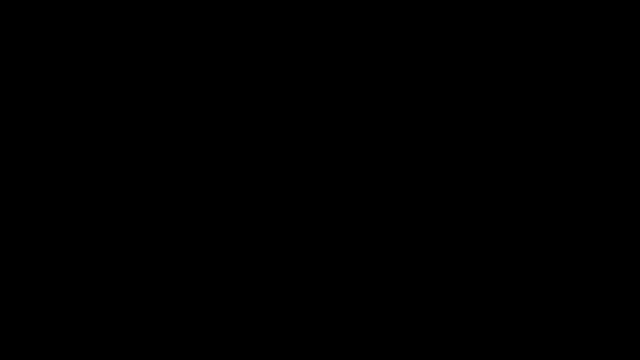 How about some radium Want to tell the time? How about some radium Want to get down funky? Oh yeah, yeah, Radium, Radium will do the trick. Whoops, the positive energy is giving everyone a case of decaying alive. 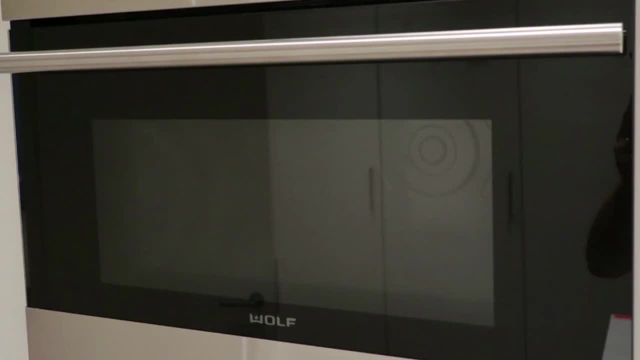 Actinium, Good for shooting neutrons. Thorium, Used in TIG welding Microwaves and in glass Protactinium- Useless, And I'm not I'm not saying this to be mean This element is genuinely useless. 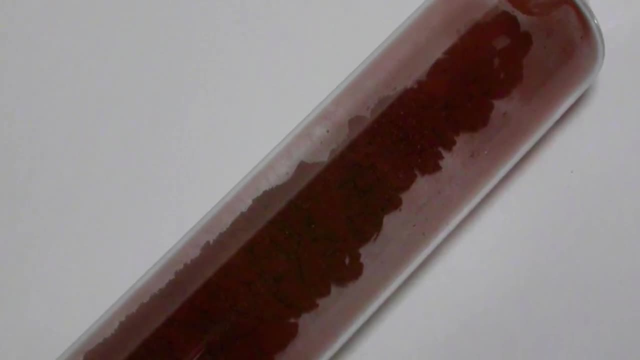 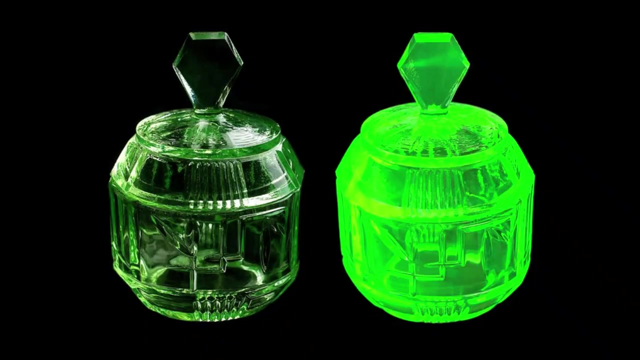 It's extremely toxic, very radioactive, And protactinium's name literally comes from the names Proto-, Actinium, Actinium. His name isn't even original, It comes from Actinium Uranium Reactors, Glass, Intercontinental ballistic missiles. 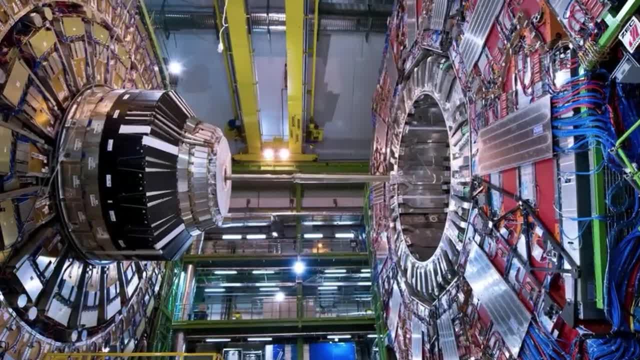 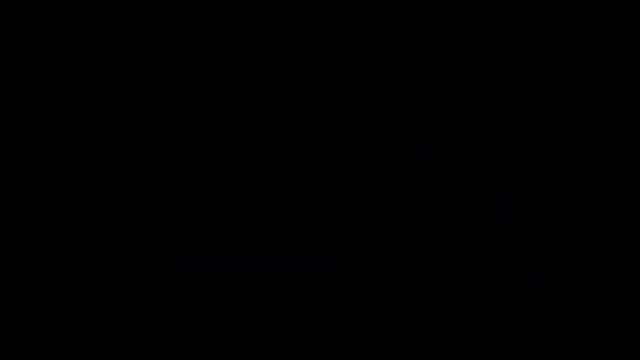 Dentures, Neptunium- He's also used in firing neutrons, so I guess he gets a pass- Plutonium, Nuclear batteries, Americium Smoke detectors, Curium Rovers and other spacecraft Also at this point forward. owning any of these elements is illegal. 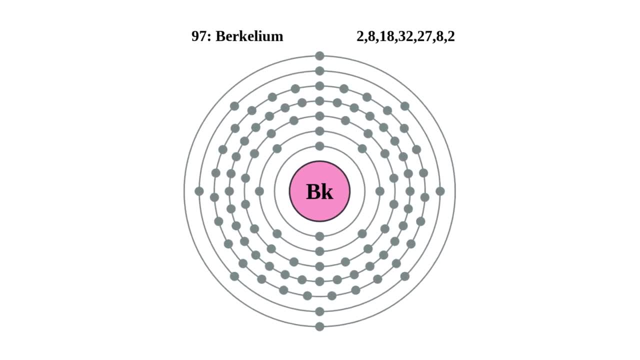 Brachylium Berkelium Berkelium. This one's used in creating super heavy atoms on the periodic table. I've always wanted an element called metanarium Californium. Want to know how moisture oil Soil. 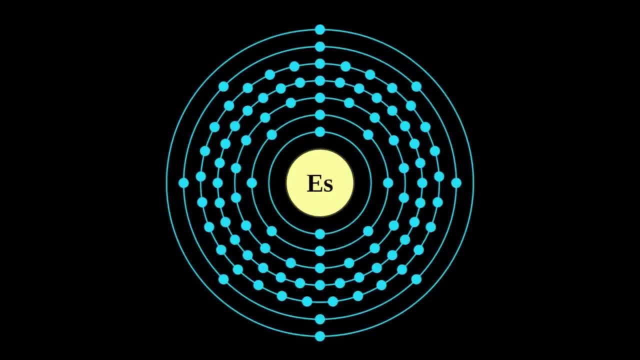 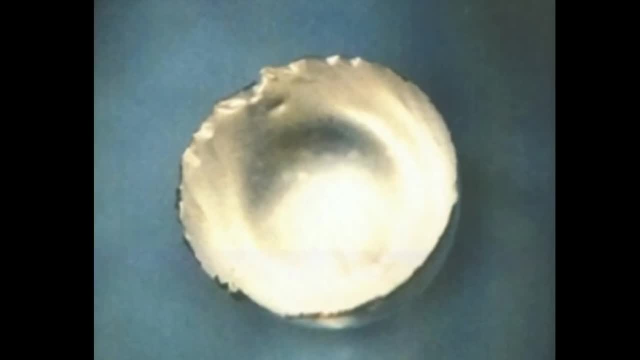 Or foil, is You do Cool, Einsteinium? This one glows blue Just from extreme radiation And I find that super hilarious Fermium Used in alloys to figure out the enthalpy of vaporization of itself. He's trying his best.